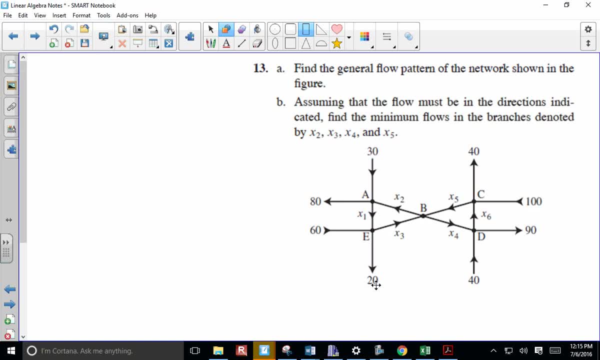 Anyway, we know that input and output have to be the same, So we go by intersection or indicated point. I guess there could possibly be more intersections than are actually indicated. We have A, B, C and D. Don't get put off by the nature of the diagram, because you know like I mean. I 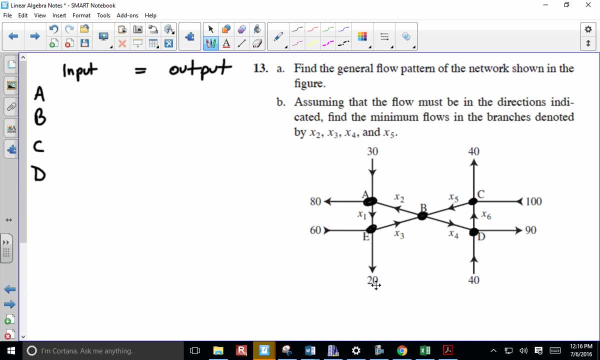 could. I could throw one at you that has an ellipse in it. You know, it really doesn't matter what the angle is and that you're approaching the intersection, just matters what the value is going in and what the value is coming out. So it could be an X formation like this. Maybe we have just a. 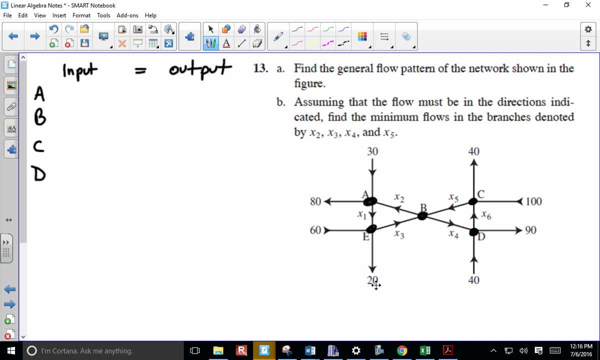 simple T intersection. Maybe we've got a circular like a roundabout kind of thing, like over by Kensico. You know, the foundation of a technology assignment We'll get there. So at A you look at the arrows that are coming in, We got a 30.. 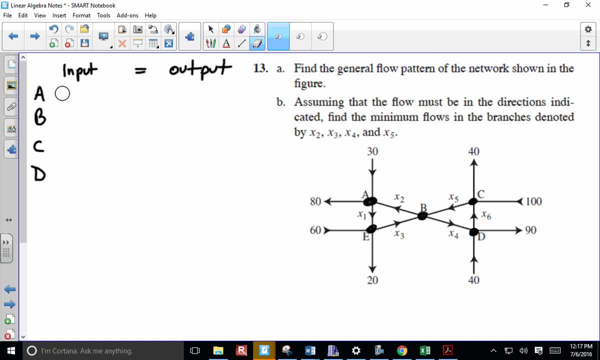 I'm gonna go with this smaller. we have an X2.. On the output, we have an 80 and an X1. And input and output has to be the same, otherwise the network fails. At B, we're coming in. at X3 and X5. We're. 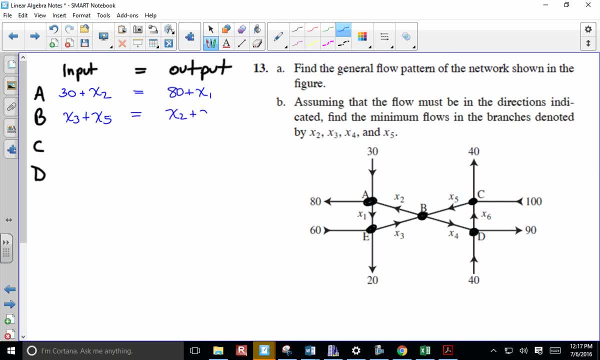 coming out at X2 and X4.. C, we're coming in at 100 and X6.. We're coming out at X5 and 40.. And D, we're coming in at X4 and 40.. Coming out at X6. 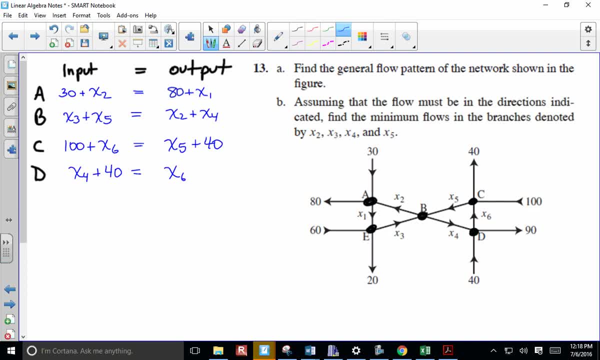 6 and 90. you just want to make sure that you've accounted for every possible pairing, not even pairing, I don't know why I said that. I just grabbed the word and threw it out there. every value that you see listed on here should be represented in your network in some way, so so I'm missing something. yeah, because 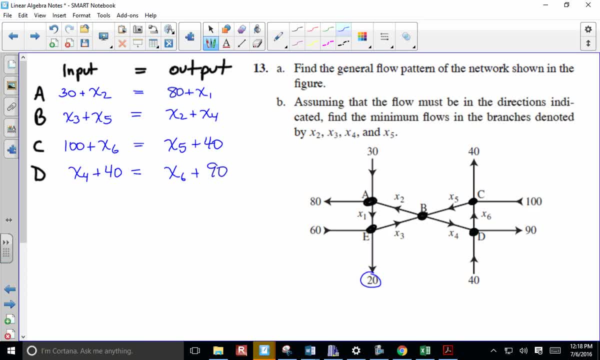 I was looking at, I see a 20 there as like I don't have a over 20. so at E we have 60 and X 1 and coming out X 3 and 20. they just do a quick look around, make sure everything's accounted for. that's all, all right. 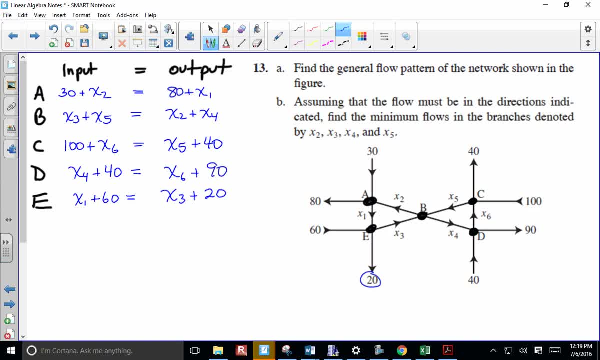 we'll. we'll get to the, the matrix aspect of it, but just get a sense of what the question is asking, assuming the flow must be in the directions indicated. so that means that if you get- we talked about this yesterday- if you get an X 2. 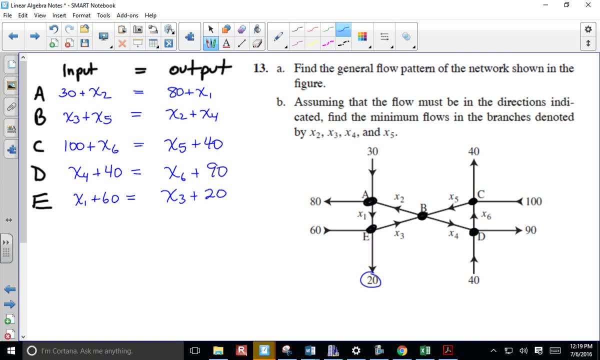 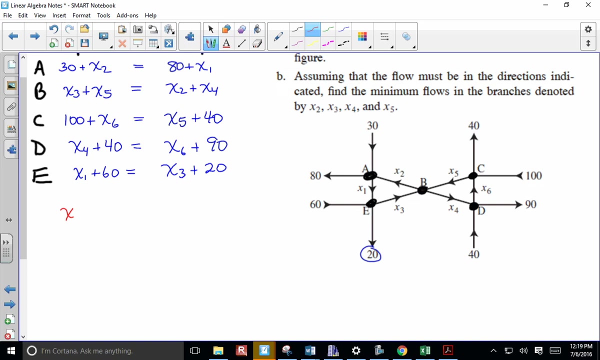 that's negative. that means it's going in the opposite direction. you did something wrong, all right, so so yeah, find the minimum flows in the branches denoted by man. all right, so homogeneous equation. we're looking at X sub 1, which way we want to bring it. I guess we're bringing 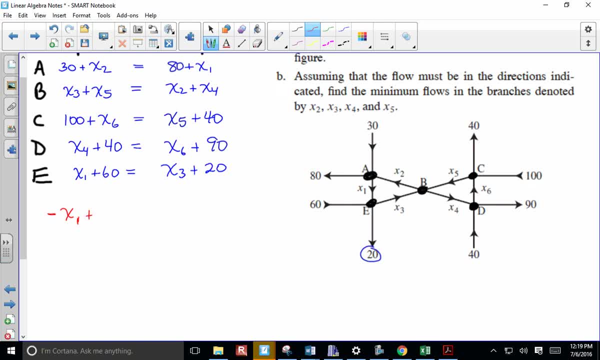 it the other way, so negative X sub 1 plus X sub 2. we don't have a 3, 4 or 5, so you could skip it if you want, or you could write: plus 0 X of 3, plus 0 X of 4. 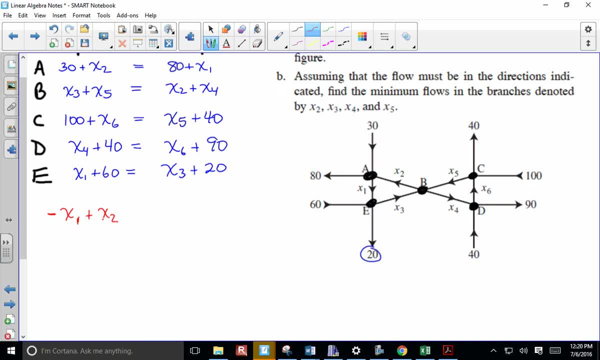 plus 0 X of 5. I'm going to be tight on room. some gonna skip that part of it and make it a 50 on the right. we subtract 30, it looks like everything's going to the left and the zero is gonna remain on the right. 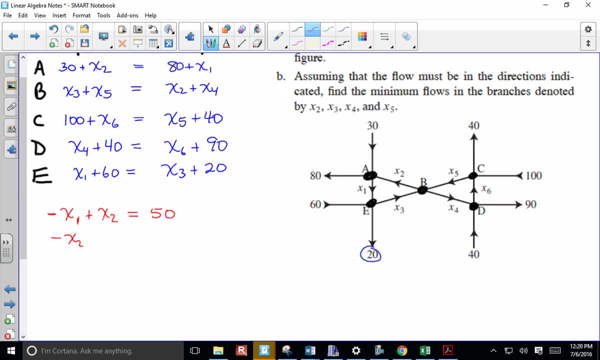 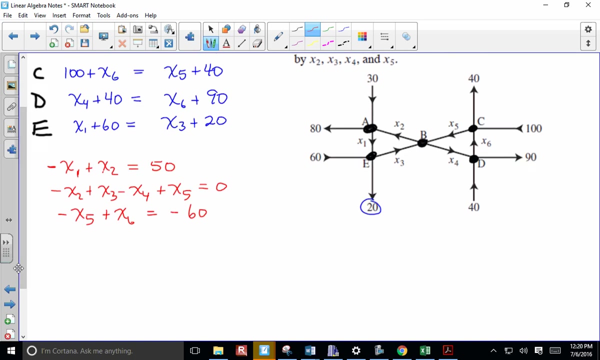 for B. so negative X to the X 2 plus X 3 minus X 4 plus X 5 equals 0. negative X 5 plus X 6 equals negative. 60 X 4 minus X 6 equals 50. X 1 minus X 3 equals. 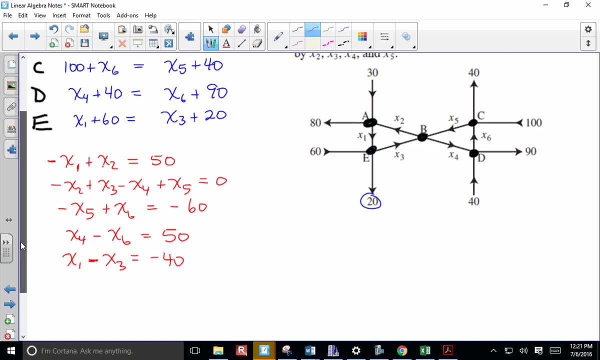 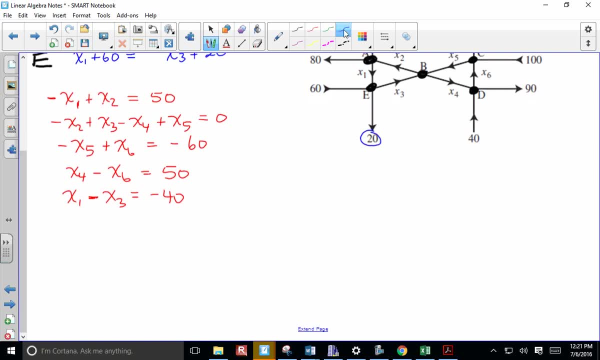 negative 40. stop me if I botch that, but I think it's looking pretty good. all right, we'll go to our matrix equation, which would be negative: 1: 1. then 3, 4, 5, 0. negative 1: 1. negative 1: 1. 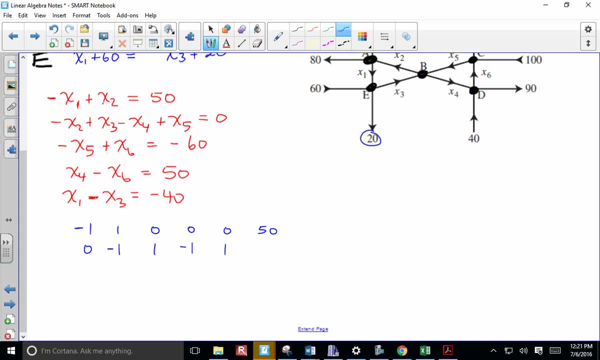 oh, and a 50 at the end, of course, 50 and a 0. yeah, 0, 0, 3, 4, 1, 2, 3, 4. I think I'm missing something. 3, 4, 5 on the first one, on the first row, extra zero. 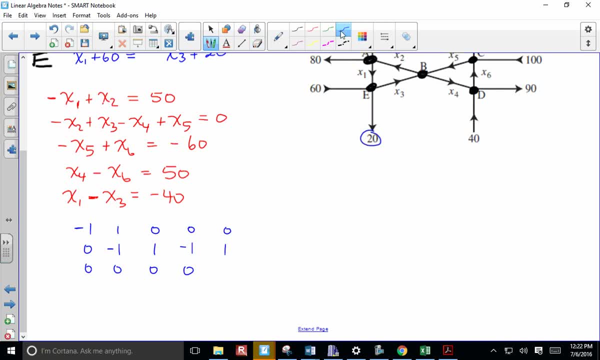 oh yeah, because it goes to 6, not 5. okay, gotcha, all right, so then 0, 0 and 1, 2, 3, 4 negative, 1 1 negative 60, 1, 2, 3, 1 0 negative 150. and. 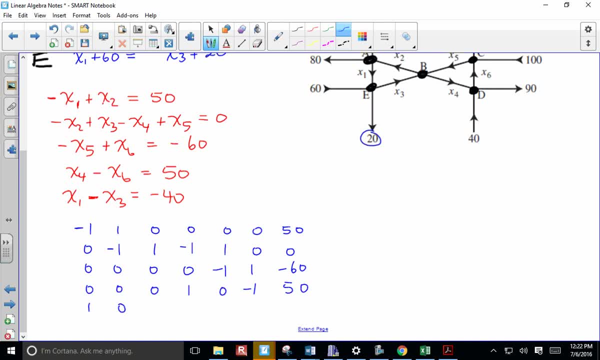 and 1,, 2,, 3, 0,, 0, 0, negative 40.. All right, So that's our augmented matrix. And just again, if the question tells you to be sure to write the, write it in matrix equation form. first, make sure you do that. 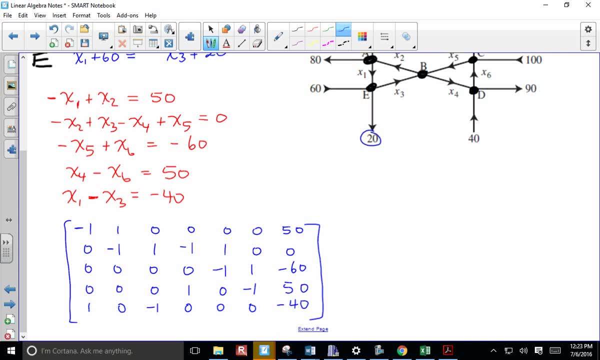 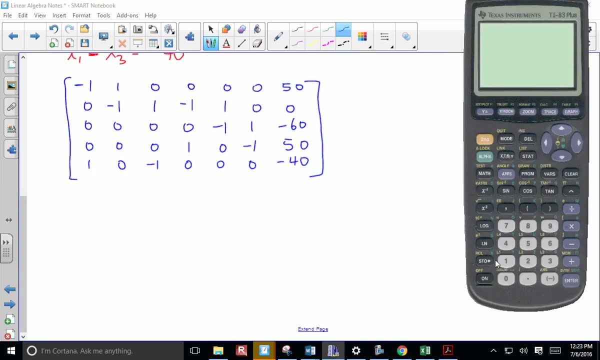 AX equals B, So coefficient matrix times the column of X1 to X6 equals 50, 0, negative 60, et cetera, et cetera. All right, This is a. this looks like it wouldn't be too bad to do by hand. 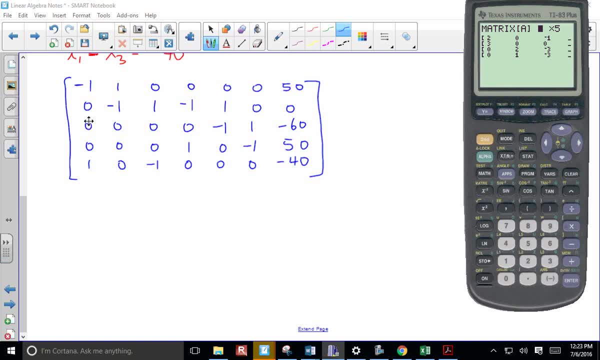 But I'll tell you the same thing. I told the guy when I was writing this. Okay, When I was buying the air conditioner yesterday, he said: you want to just throw it in the car? Save you $100 on delivery and installation. 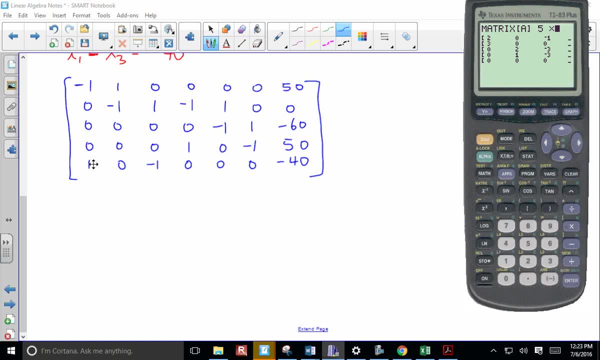 And I was like, no, He's like you sure. I was like, yeah, I'm sure Why I don't want to. I just I don't want to do it. So you're going to do it. 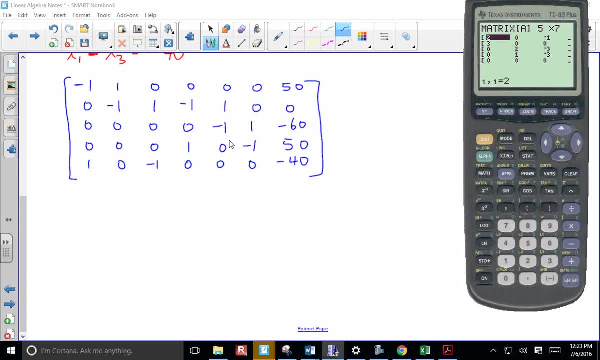 And so that's the idea here. I don't want to do it. I just don't want to do it by hand. So I'm going to mindlessly type it into the calculator and let the calculator do it, And I'm not even going to pay it. 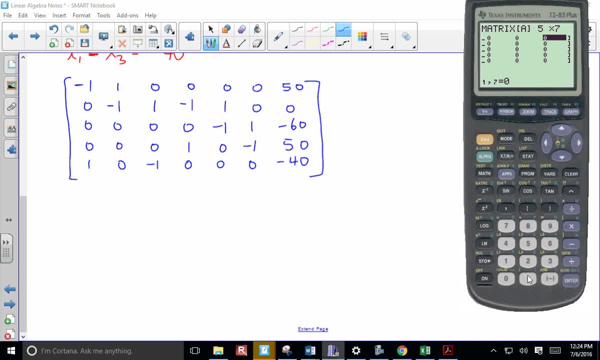 Of course. that being said, it's almost after that whole spiel. it's almost like a preordained requirement that I'm going to screw this up. Nothing will shake your confidence, quite like a course on linear algebra. You're like I got it. 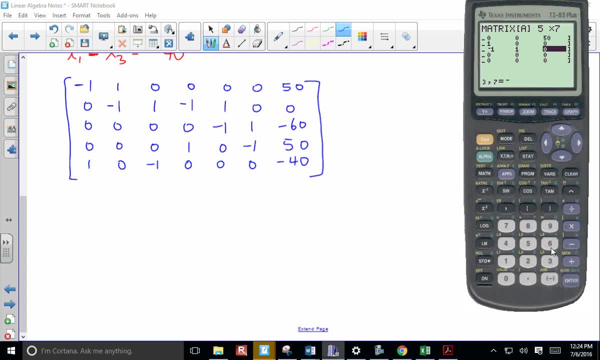 Totally nailed it. No, You screwed something up. I think I typed it in right. Got to say, though, I no longer care, Because after that I got to do a, I got to do a double snip here. 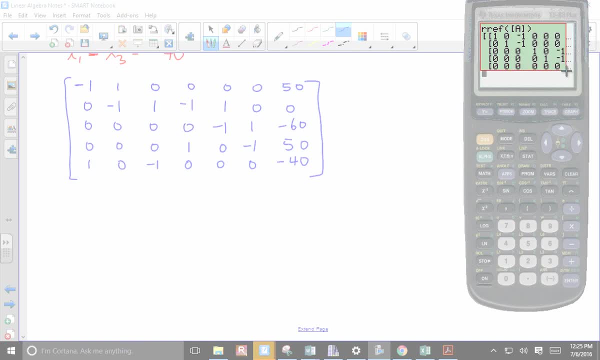 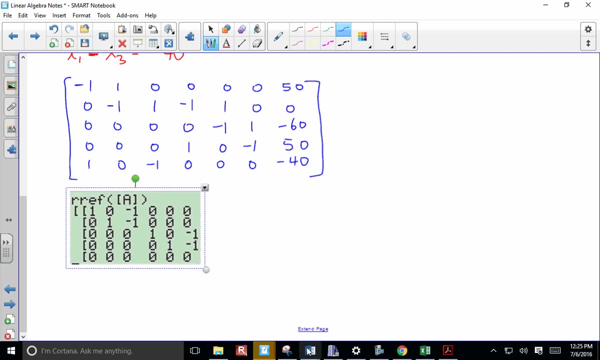 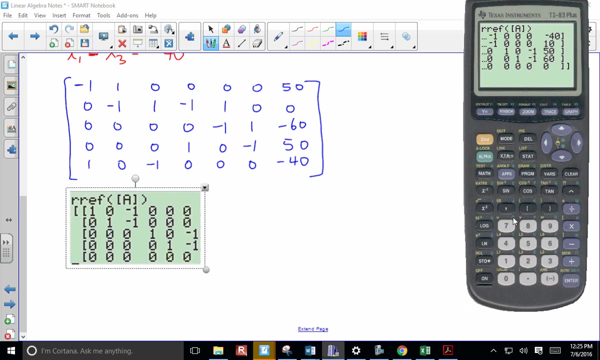 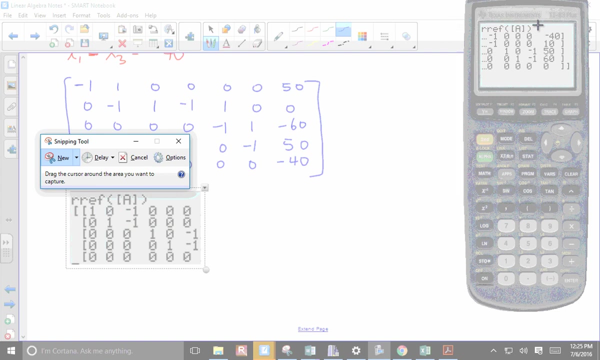 It always was So annoying, Jesus So busy. let me sneak this in. Get on out. 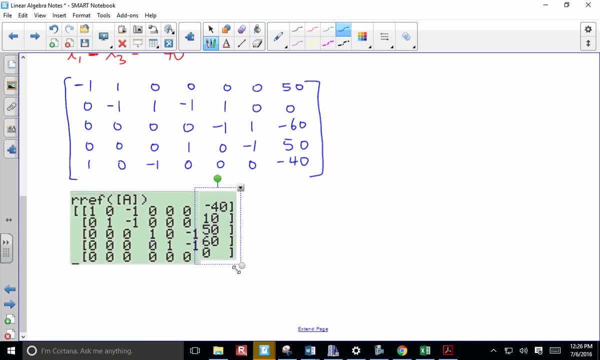 Oh, that looks like a negative 150,. all right, okay. so again we're looking at X1,, 2,, 3,, 4,, 5, and 6, so X1 would be equal to negative 40 plus X3, or X3 minus 40, however you like. 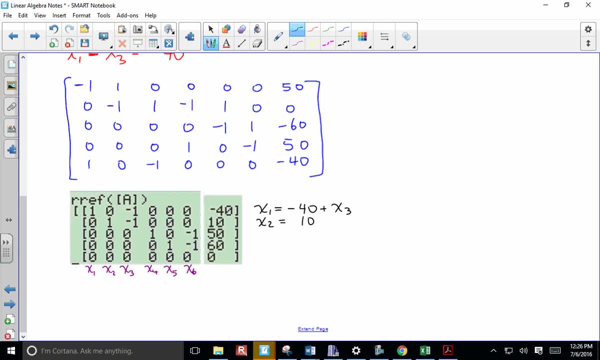 X2 would be equal to 10 plus X3.. Now X3 is not represented right in terms of a pivot, so we'll come back to that. X4 is equal to 50 plus X6, X5 is equal to 60 plus X6, X6 is equal to 60 plus X6, X3 is: 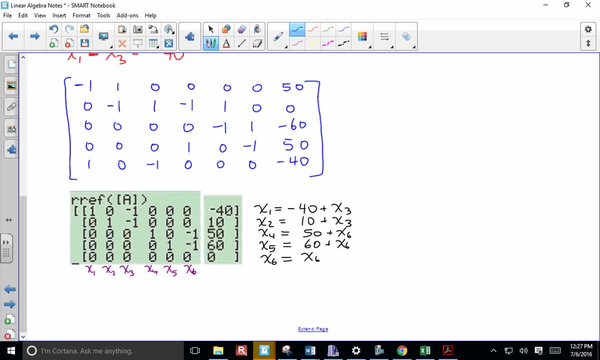 equal to 50 plus X6, X3 is equal to 60 plus X6, X3 is equal to 60 plus X6, X3 is equal to 60 plus X6, and so you know what happened to the X3, also a free variable, so you can. 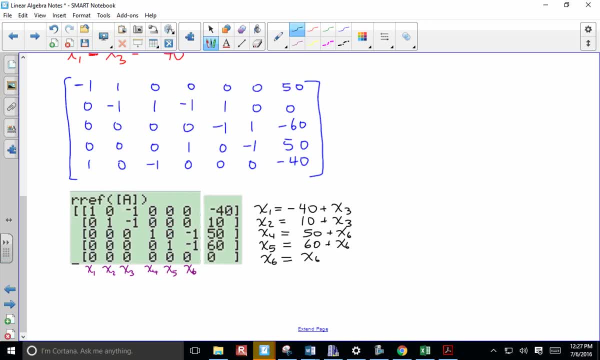 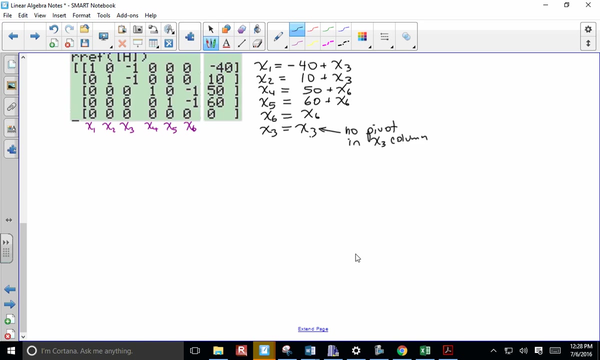 tuck that in if you want, or you could just say: X3 is free, however you want. all right, so X3 equals X3,. all right, and that's because there is no pivot in X3, so X3 is free. all right, so X3 is free, all right, and that's because there is no pivot. 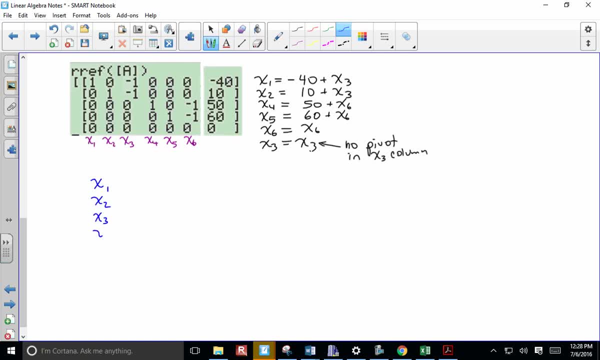 in X3, and so you know what happened to the X3, also a free variable, so X3 is free. all right, so we go to parametric form and I would say that that should be your go-to in terms of how to represent a final answer. 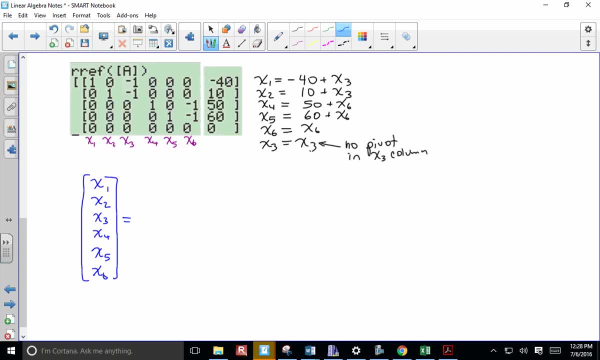 Or at least get you to the final answer, because more often than not it's going to serve the purpose. but even if it's not precisely what's needed, it will at least get you kind of going in the right direction. Constant values: we've got negative 40,, 10,, 50.. 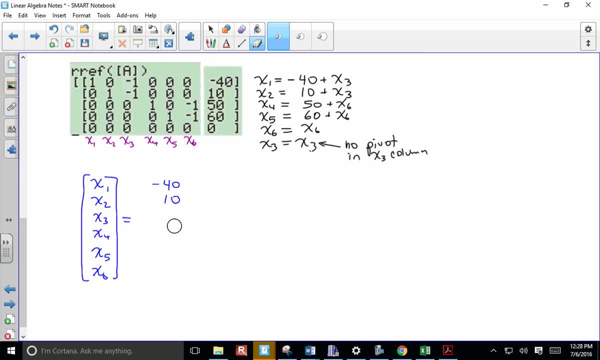 Now you see I'm going to screw myself up here. now The 3 comes in there, Alright. so negative 40,, 10, a 0 for the x of 3,, 50,, 60, and a 0 for the x of 6.. 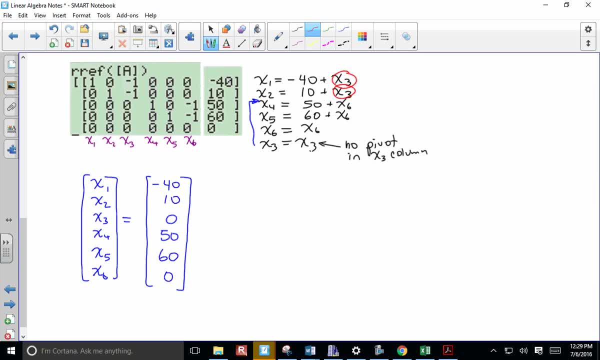 Alright, our variables. here we're always writing it in terms of the free variables. So we're going to need two pieces to our parametric. So we're going to need one for the x of 3. And we're going to need one for x of 6.. 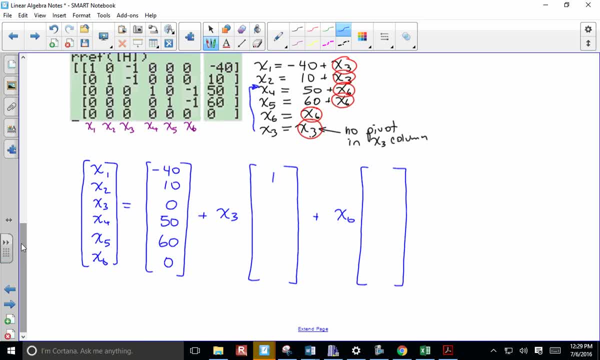 So for x of 3 we have coefficients of 1, 1.. For the free variable, For x of 4 there's nothing. 5 and 6 there's nothing. For x of 6, we have nothing in x of 1, nothing in x of 2, nothing in x of 3.. 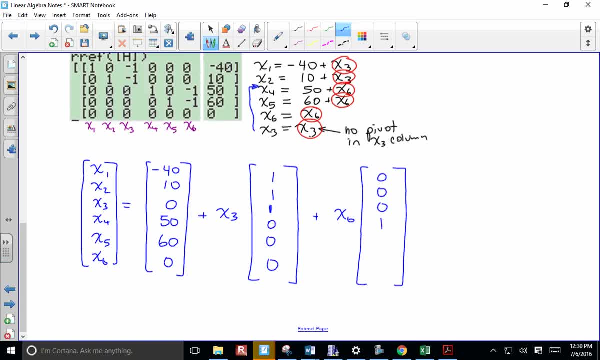 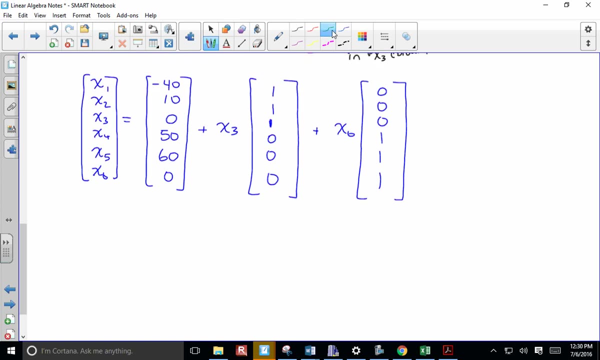 In x of 4, we've got 1x of 6, same thing with 5. And 6.. Alright, now just a little vocabulary here. not really vocabulary, it's just how it ties together. You might remember the formula w in parametric form: w equals p plus vh, and so this is the 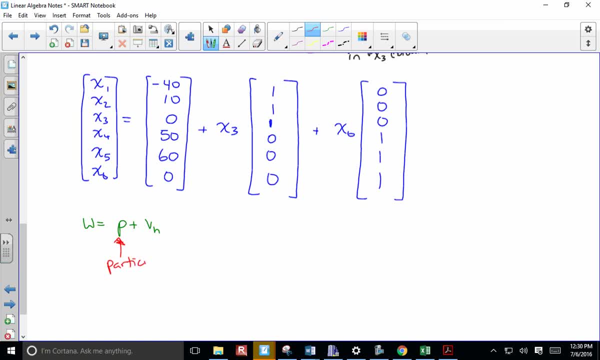 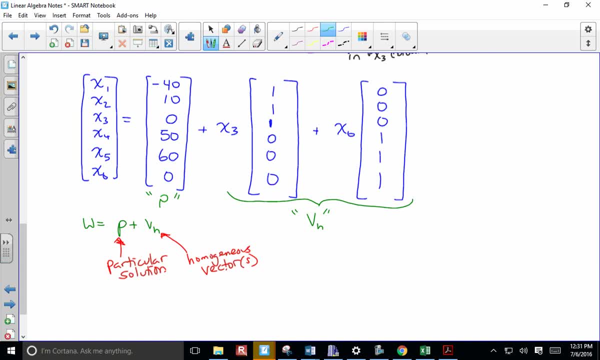 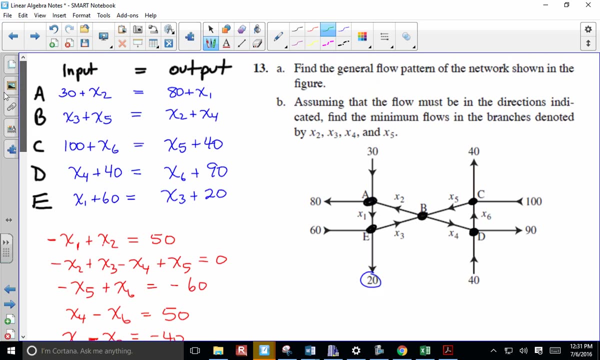 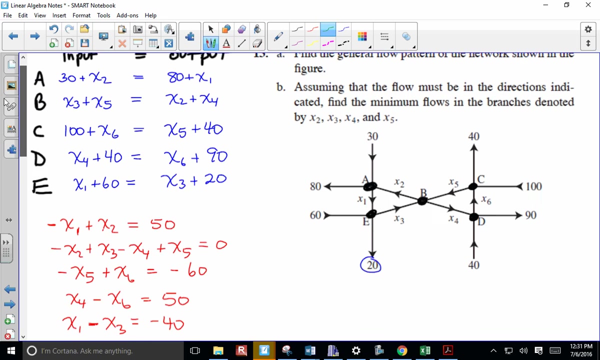 just to tie it together with the formulaic notation. but we do need something that allows us to determine the true weights. so just following the question says: assuming the flow must be in the directions indicated, find the minimum flows in the branches denoted by x2,, 3,, 4, and 5. 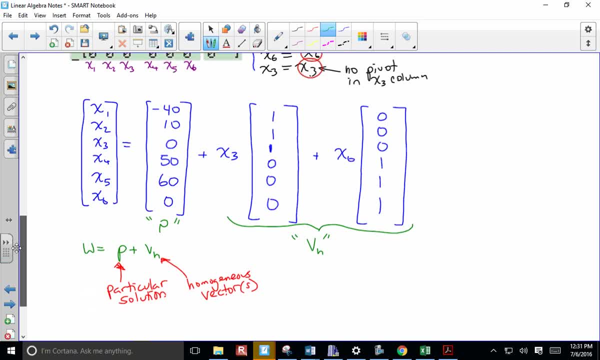 alright, so we have to address that component of it, and the issue here is the negative. we don't want a negative. so if we know that x sub 1 is going to be equal to negative, 40 plus x sub 3 and really just plus x sub 3, right? 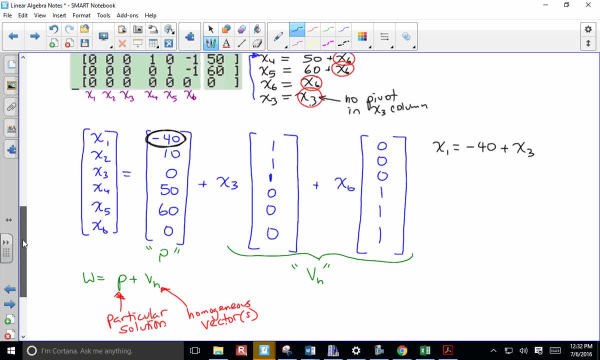 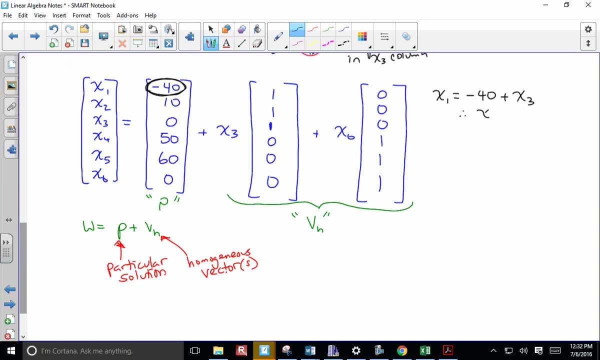 that's based on what we had up above, but also based on the parametric, because anything with a value of 0 is going to zap away. so therefore, x sub 3 has to be greater than or equal to 40, right? so, if we're assuming? 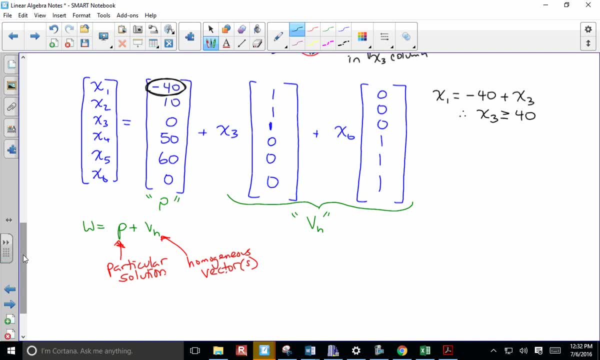 that it's a minimum value of 40, then that allows that actually allows us to go further with this if we wanted to. but we still don't know. x sub 6. really, all I need from you is to really state what the minimum value would be in order to make it a positive measure. 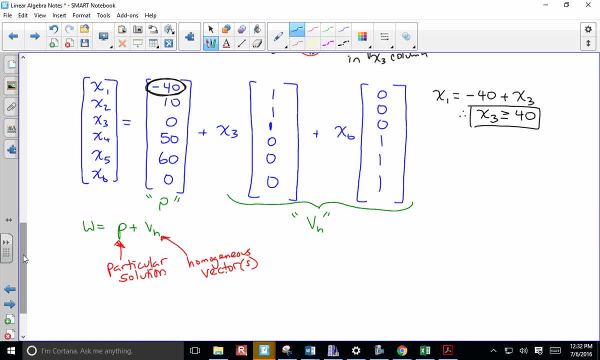 because beyond that it really doesn't matter what. x sub 6 is a free variable, but x sub 3 has to be at a minimum. x sub 3 is free also, but in order for it to satisfy the network it has to be at a minimum of 40, otherwise everything falls apart.